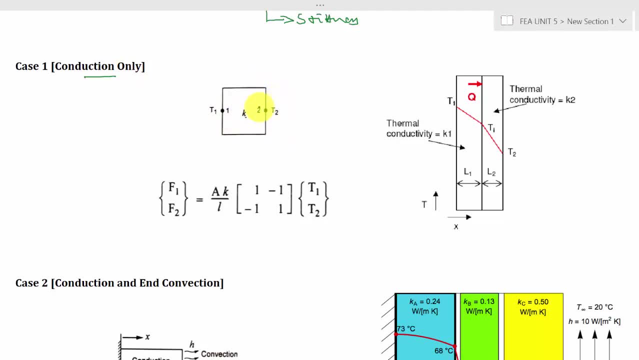 only conduction, that is, the element is insulated throughout, because we have three modes of heat transfer: One is conduction, the second one is convection and the third one is radiation. So in FEI we will have conduction, convection and internal heat generation when the body is insulated in the surface. 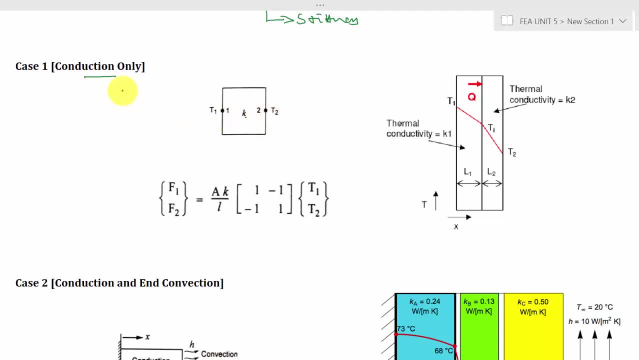 and it is subjected to conduction alone, then it comes under case 1. so if it is subjected to conduction, then we have a higher temperature at the node 1, and when the conduction takes place, I mean thermal conductivity will be given, so the temperature of node 2 is reduced. 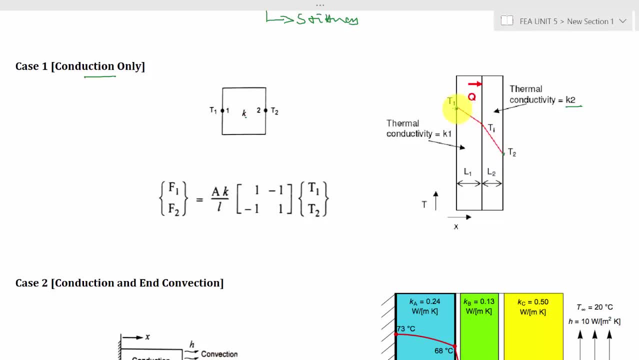 because of the conduction losses, The temperature is transmitted to T2, so T1 is reduced to T2.. So the FVA equation for calculating conduction is: F is equal to K into T, so here F is the force vector. If F is the force vector, right. 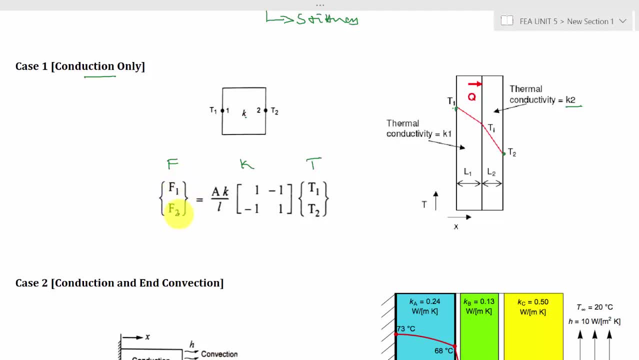 any external load is applied. then we can consider F1 and F2.. Then K is the stiffness matrix for conduction. So here the equation is Ak by L. Here A is the area, cross sectional area, The K is the thermal conductivity, Then L is the length of the element, Then T1 is 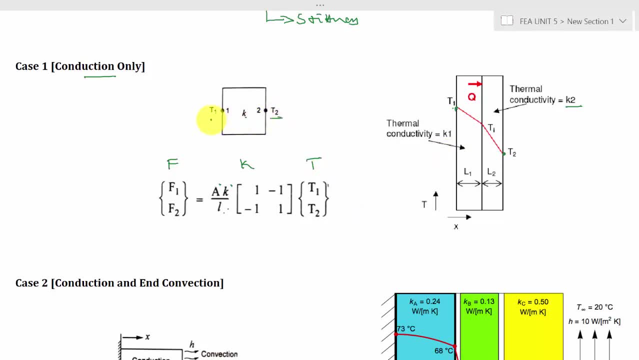 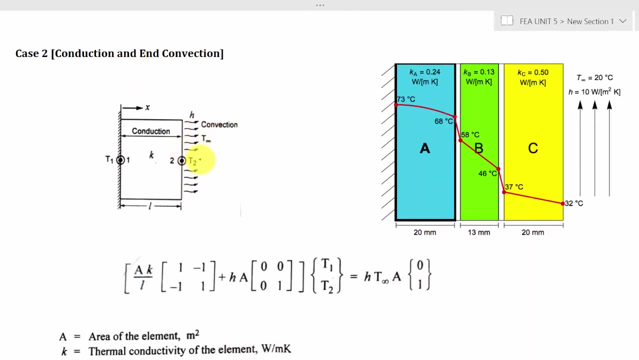 the temperature at node 1 and T2 is the temperature at node 2.. So if the cross section area is not given, then we can consider a unit cross section area. The second case is conduction and end convection. So here the end is exposed to atmosphere with some heat transfer coefficient. 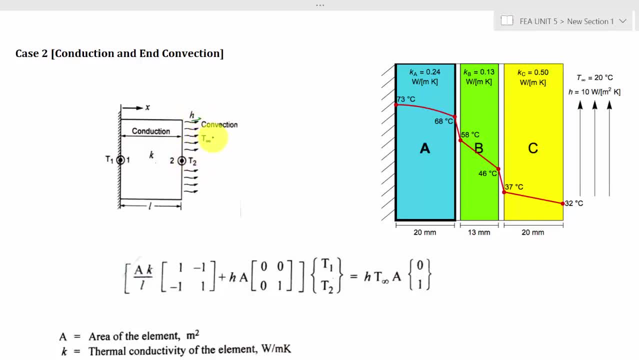 The H value will be given Here. the ends are not insulated. That is why it is exposed to atmosphere. So throughout the section it is subjected to conduction and at the end it is subjected to convection. So that is the second case. 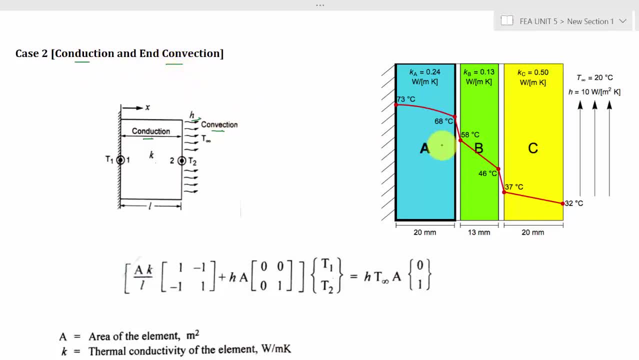 So conduction and end convection. So here I have considered 3 elements. This is element number 1, element number 2 and this is element number 3.. So the node 1 is subjected to only conduction, I mean element 1.. The element 2 has only conduction, The element 3 has both. 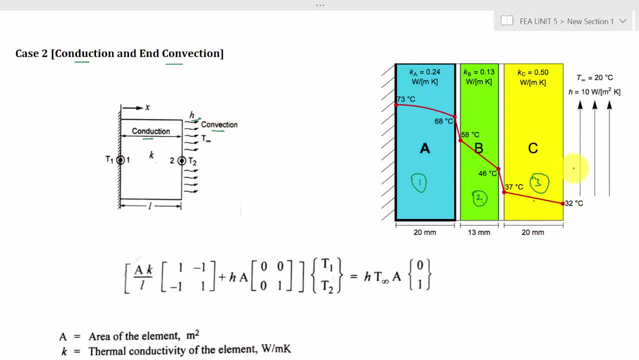 conduction as well as the end convection. So this comes under case number 2.. So mostly volts problem comes under case 2.. So this is the equation for conduction with end convection. It is Ak by L, 1 minus 1 minus 1, 1.. So this is for convection, k convection, and this is 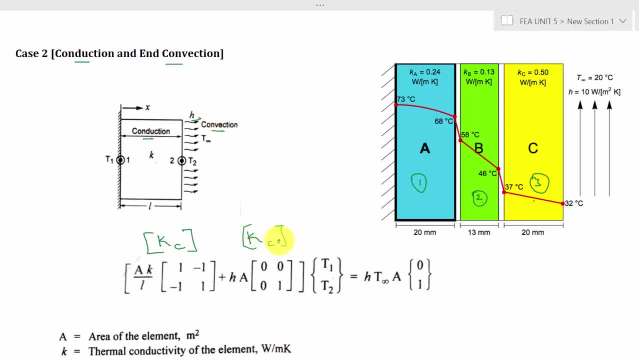 for k conduction. So this is Ha, 0, 0, 0, 1, because the conduction takes place only at the end. So here H is the heat transfer coefficient. So here H is the heat transfer coefficient And A is the cross sectional area, And here this is the force vector. So it is H, T, alpha. 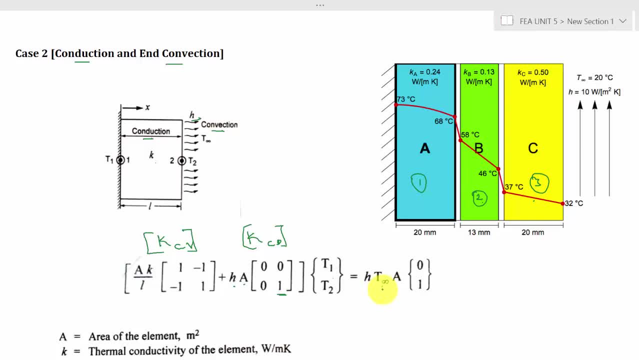 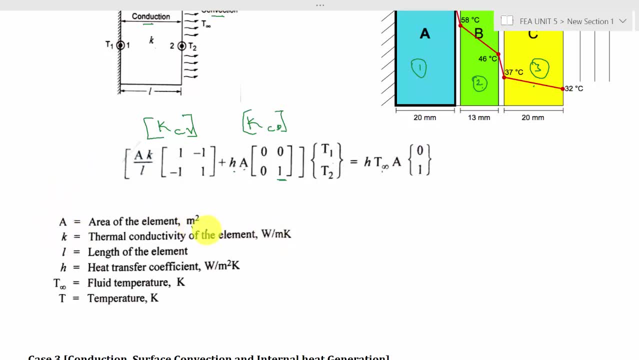 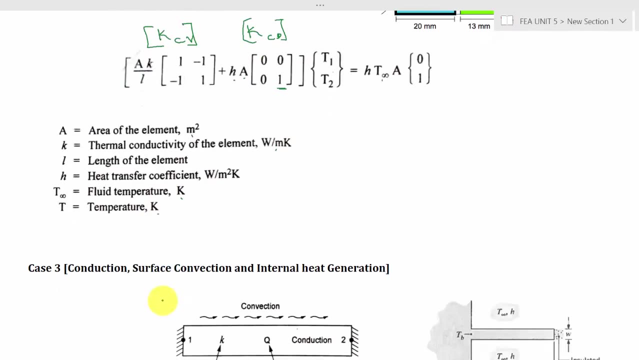 into A T. alpha is the atmospheric temperature. So these are all the units. I am going to substitute the area in meter square. thermal conductivity in watt per meter kelvin, temperatures in kelvin. Then the third case is conduction, then surface. 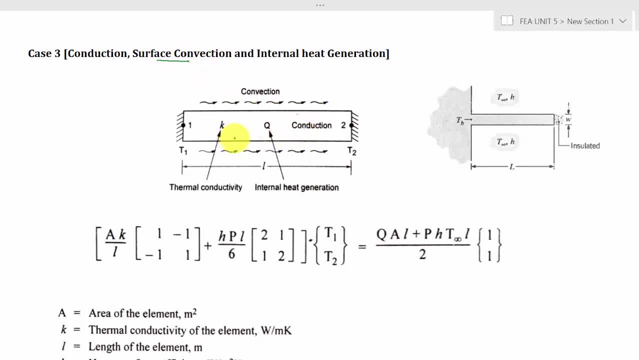 convection. So here the surface is not insulated, So it is exposed to atmospheric. So you can see the symbol. So convection takes place at the surface and the end is insulated. You can see that the end is insulated. so there is no end convection, but the internal heat. 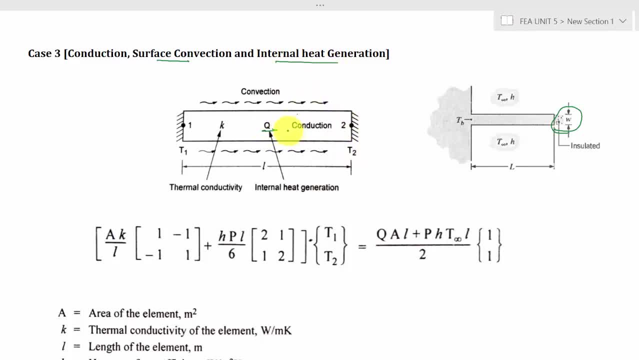 generation will be there, So Q will be given. Fine, So in case of conduction, surface convection and internal heat generation, the FA equation L, this is for k conduction and this is for k convection, So HPL divided by 6.. So here, 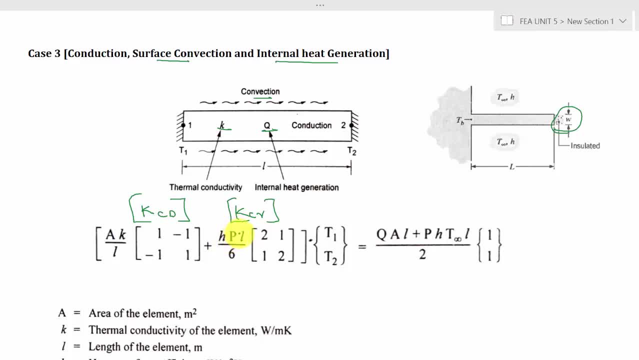 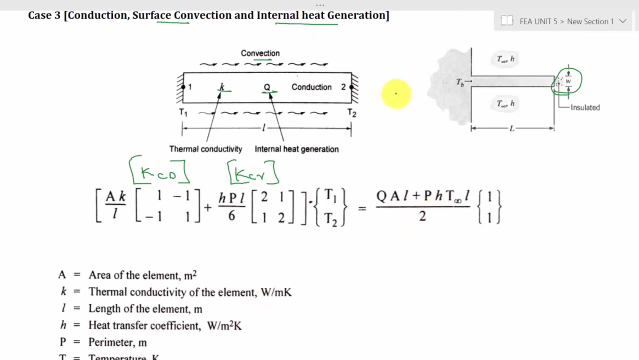 H is heat transfer coefficient and P is the perimeter L divided by 6.. And temperature. so here QAL is for internal heat generation. So here the Q is heat generation. It is given in watt and the remaining terms. we know that. So if there is no internal heat generation, 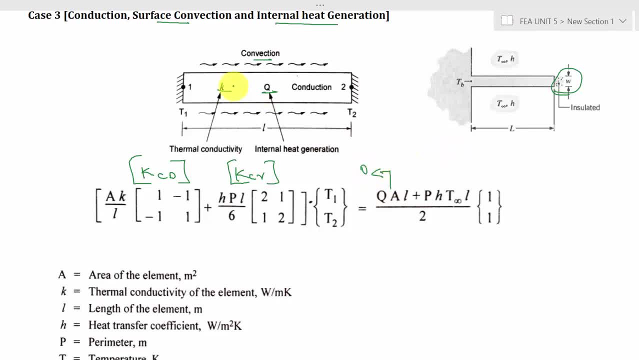 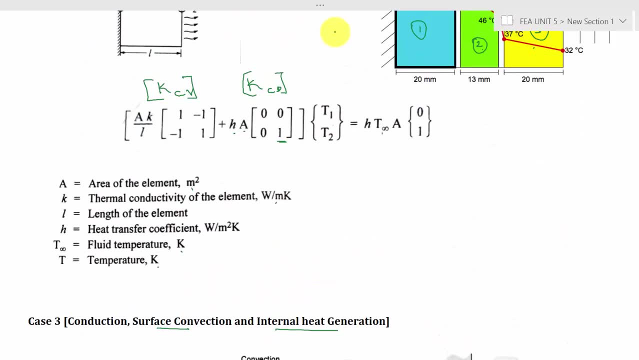 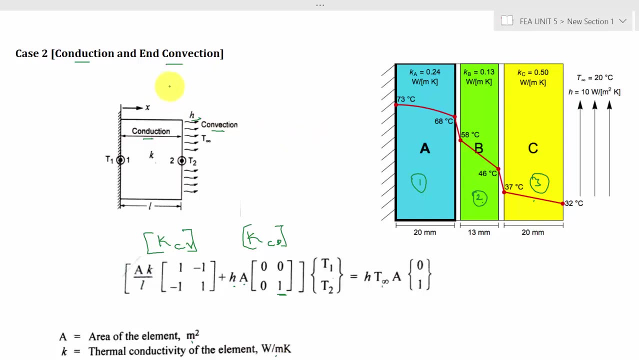 then we can put the Q value as 0. So this is in the case of conduction, surface convection and internal heat generation. So in problems we will have two types of problems. One is the composite wall problems. So the composite wall problems consists of two cases. One is 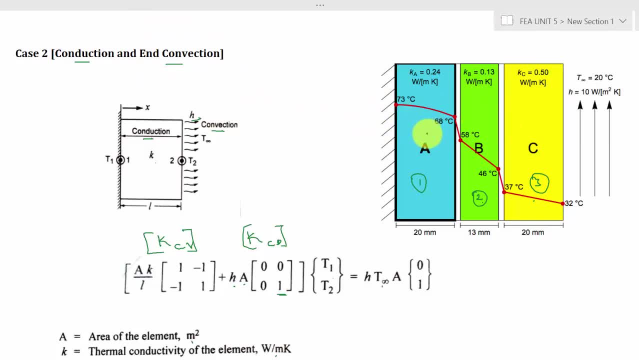 case 1, that is, this is actually the example For element 1 and element 2. it is only conduction and for element 3 it is conduction plus n convection. So this is for composite wall problems And second type of problem is fin problem. So 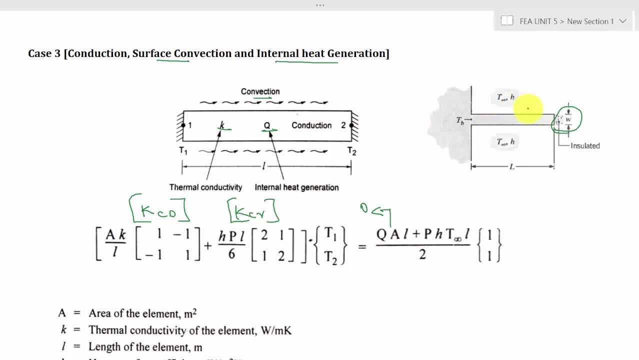 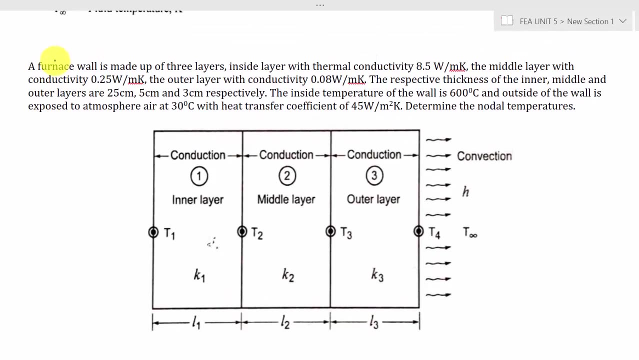 in case of fin problem you will have surface convection, So throughout the section, so you can refer case 3 for fin problems. So you have to identify whether it is case 1 or case 2 or case 3.. So this is the first problem. 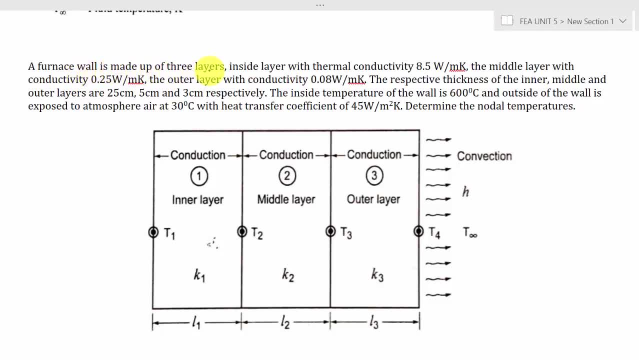 A furnace wall is made of three layers: Inside layer with thermal conductivity of 8.5 watt per meter kelvin. So this is the given drawing. Since it has three layers, I have split it into three elements. So the nodal temperatures are T1, T2, T3 and T4.. The length of the element. 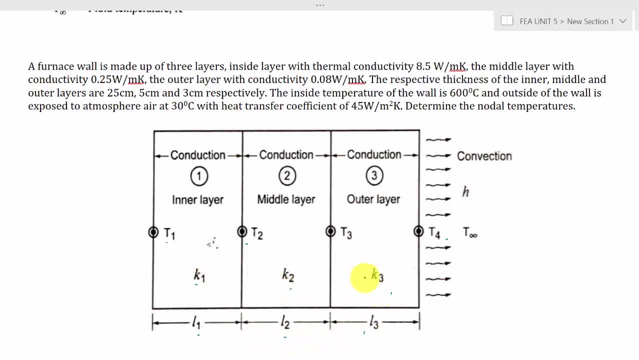 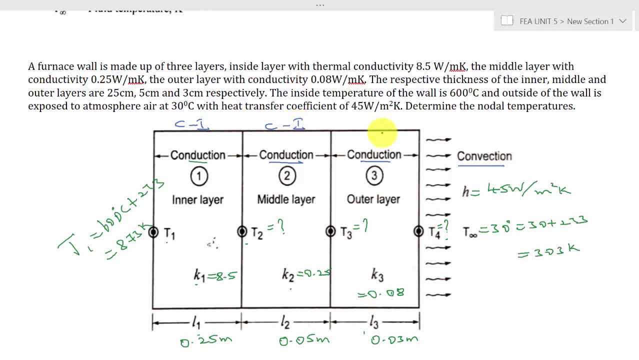 into three layers. So this is the given drawing. Since it has three layers, I have split it. For element 2, it is also case 1.. Element 3 is case 2 because it has conduction as well as the end convection, So we will start with the element 1.. So element 1 has only conduction. 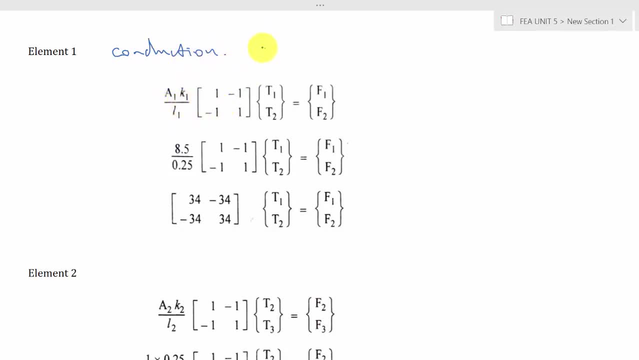 So for conduction, it is case 1.. The equation is a k by l. since it is element 1, it is a1 k1 by l1. 1 minus 1 minus 1, 1 t1. t2 is equal to f1 and f2.. 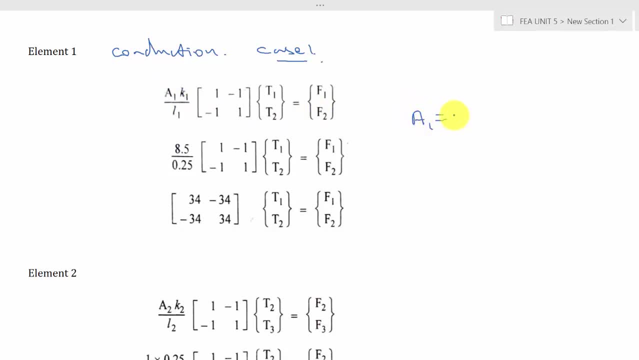 So the area cross sectional area is not given, so I am going to assume a unit: cross sectional area a1 is equal to 1 meter square k. I have substituted l1 value. I have substituted since it is given, And I have calculated the sequence. 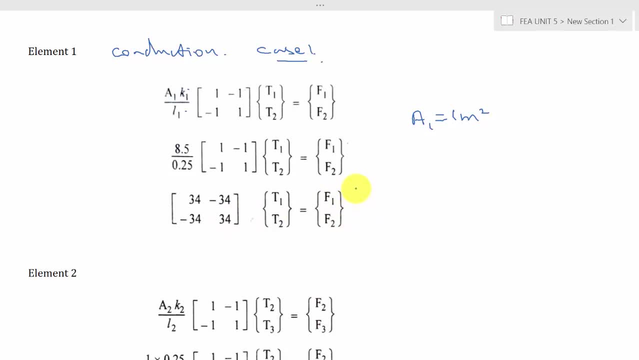 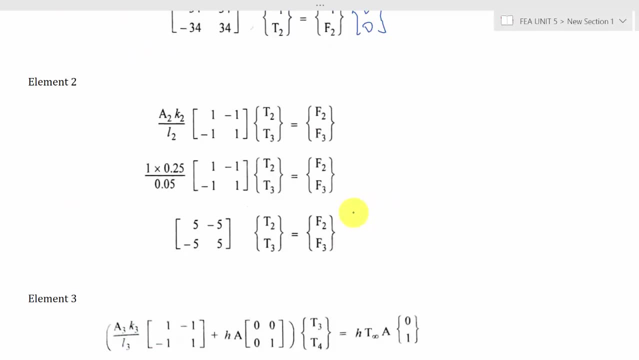 So I have calculated the stiffness matrix for element 1.. Since there is no force, external force is acting, you can put 0: 0 here. Then for element 2, it is also only conduction. If it is only conduction, then it is case 2.. 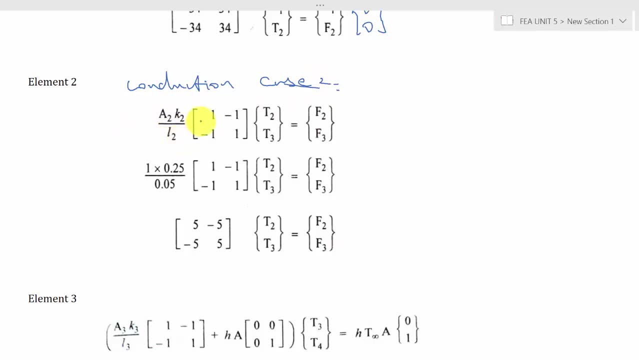 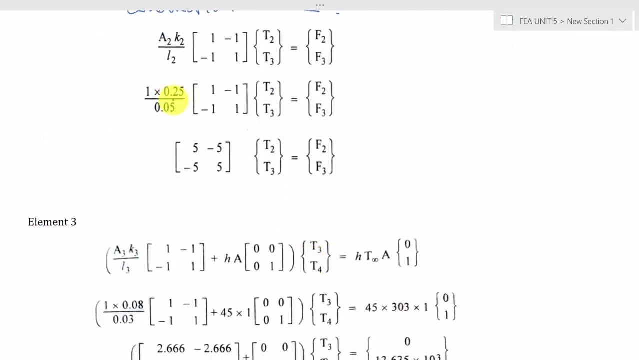 So in case of element 2, it is a2, k2 by l2, k2 is 0.25 and l2 is 0.05.. So it is 0.05.. So I am going to multiply it inside, because while assembling I have to multiply all the constant values inside the matrix. 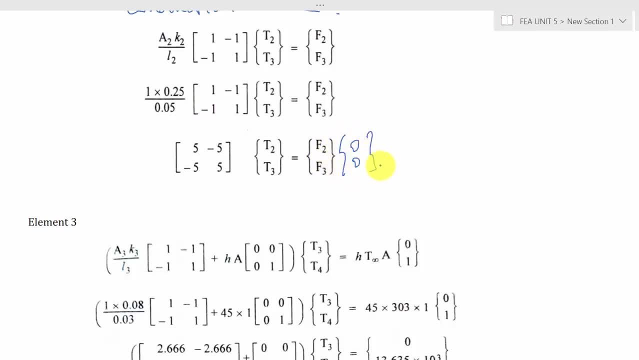 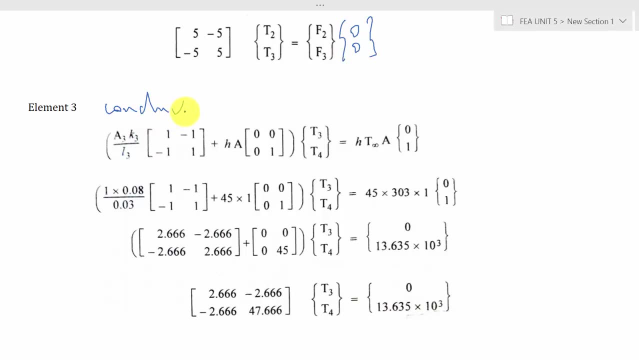 So here also there is no external load is applied, so we can put 0: 0.. Now the element 3 has both conduction plus end convection. So if it is conduction plus end convection, So if it is conduction plus end convection. 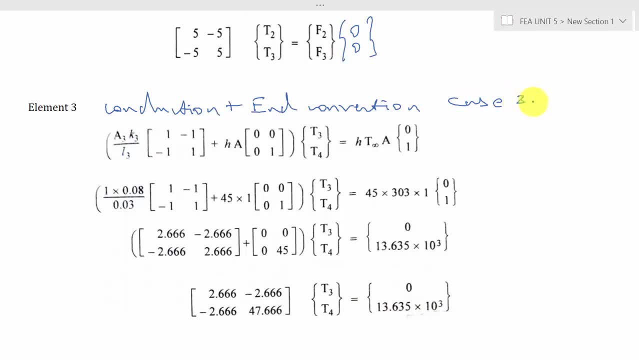 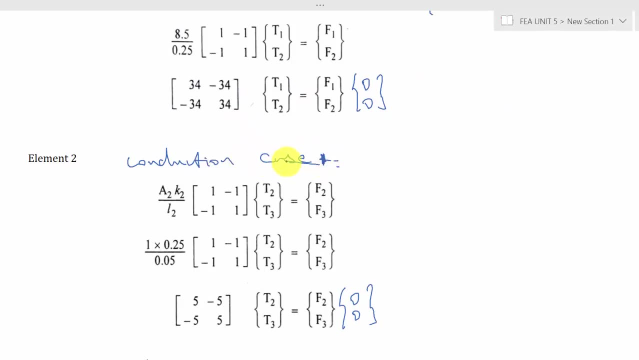 So if it is conduction plus end convection, Then it is case 2.. Sorry, here it is case 1.. Sorry, don't get confused. if it is conduction, it is case 1.. Here it is case 2, since it has conduction and end convection. 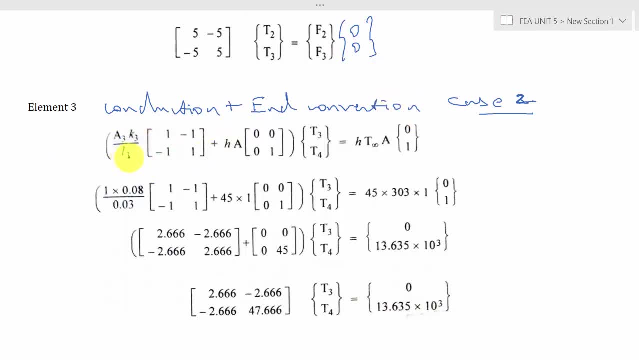 So for case 2 the equation is ak by l, since it is element 3, it is a3, k3 by l3 plus h into a 0, 0, 0, 1.. And the temperatures for element 3 is T3 and T4, H, T, alpha, A. So here A I have considered as 1, K3 value is given, L3 is 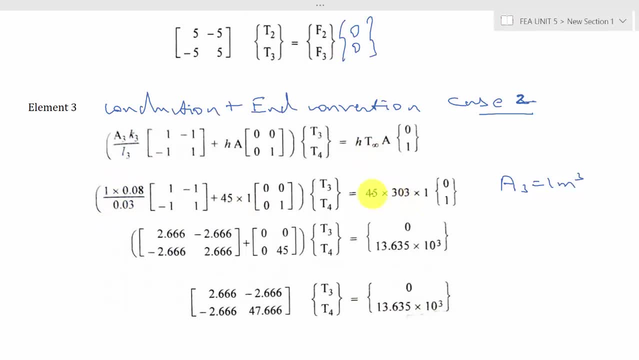 given, H is given, then T alpha is also given. So I have substituted all the values and I have multiplied it inside the matrix, then I have added these two matrices. So this is my final solution, and here I have a force vector, since it has end convection. Now, before: 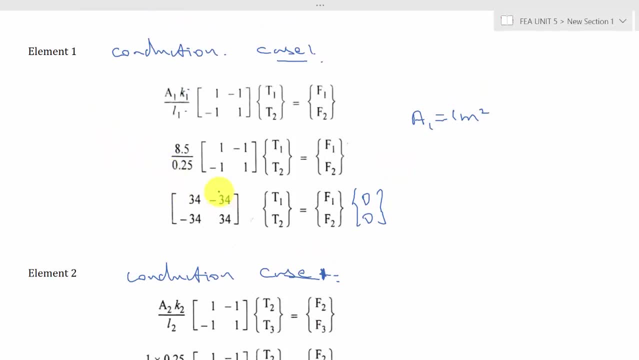 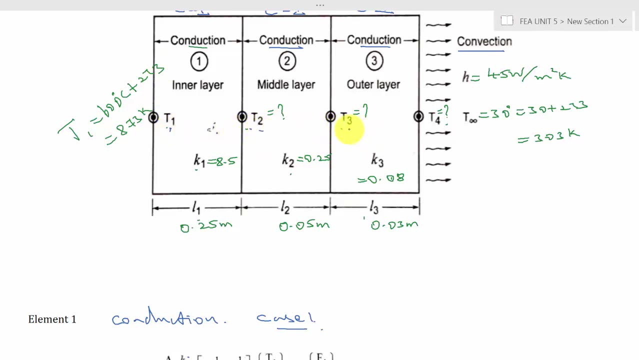 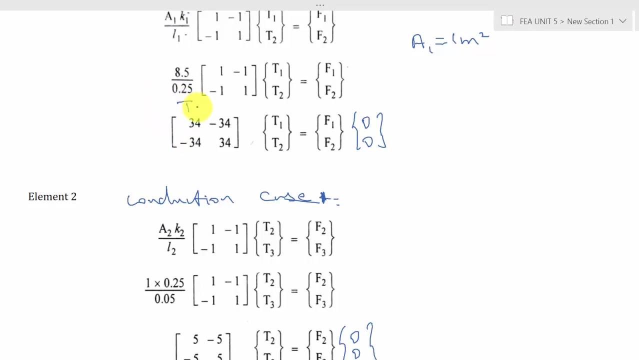 going to the assembly, I have to number the stiffness matrix. For element 1, it is T1 and T2, for element 2, it is T2, T3,. for element 3, it is T3 and T4.. So this is T1, T2, T1. 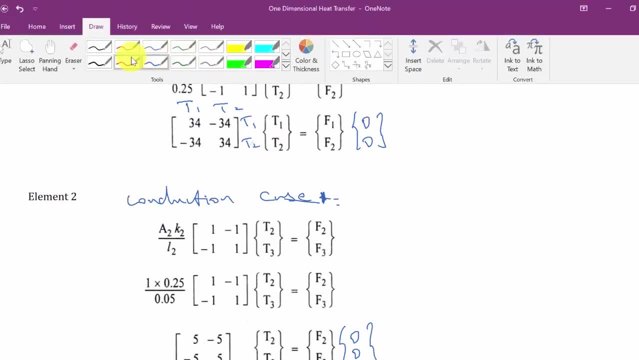 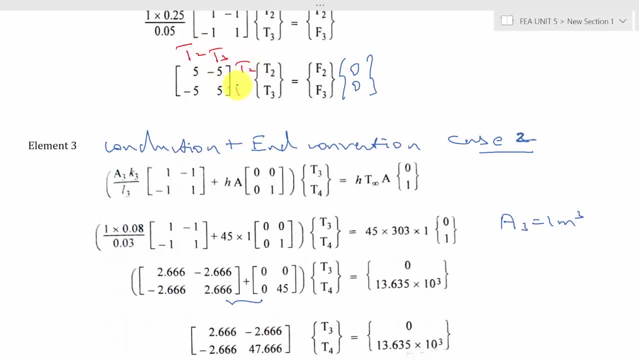 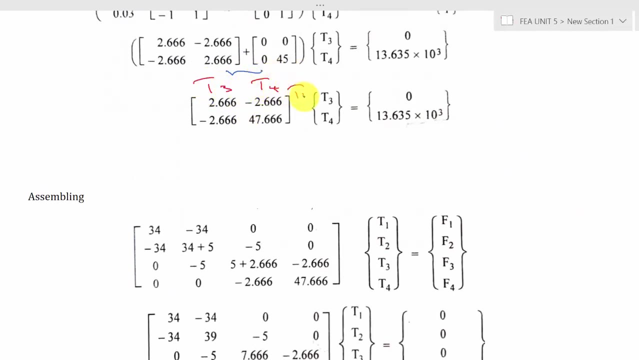 and T2, since this is for element 1.. Then for element 2, it is T2, T3.. So I have added T1, T3, T1, T2 and T3, then for element 3 it is T3, T4, T3 and T4.. So 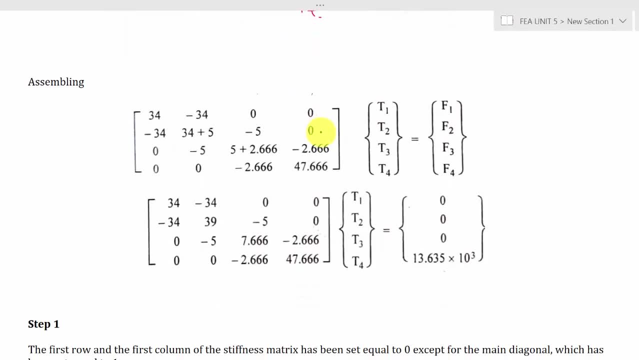 now I am going to assemble this. We know how to assemble the stiffness matrix because it is almost like one dimensional bar element. So numbering is T1, T2, T3, T4, then T1, T2, T3 and T4.. So now I have assembled all the values and this is my final solution. This. 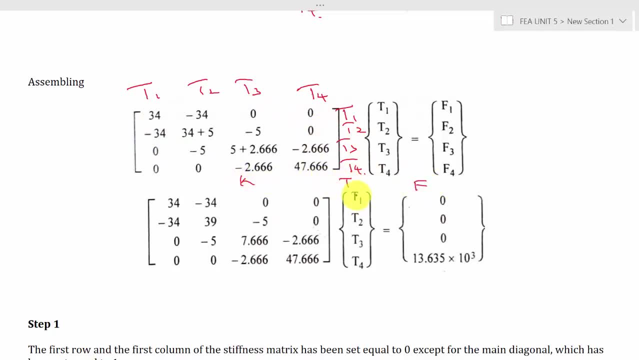 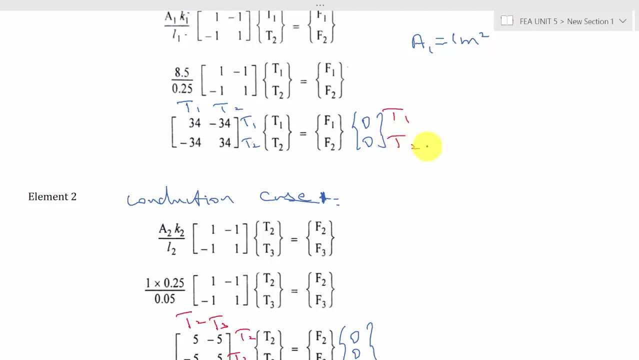 k into t is equal to f. So this is my k matrix, this is my t, and here I have assembled the force vector. So force vector for assembling force vector. also, you can give numbering. This is t1, t2, since it is element 1.. Then for element 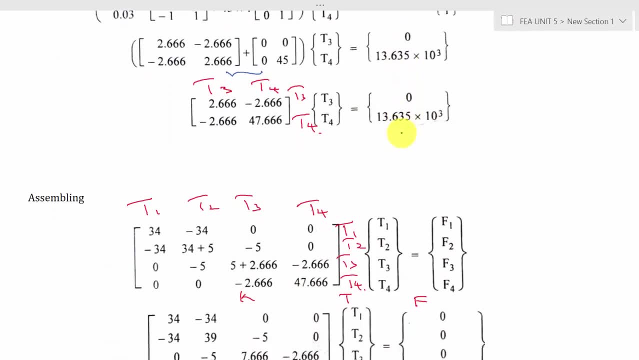 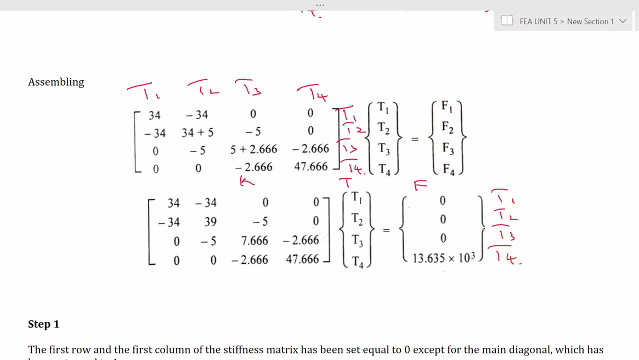 2, it is t2, t3, and for element 3, it is t3 and t4. So here it is t1, t2, t3 and t4.. So this is the final assembled stiffness matrix for the problem. So now to solve this equation. 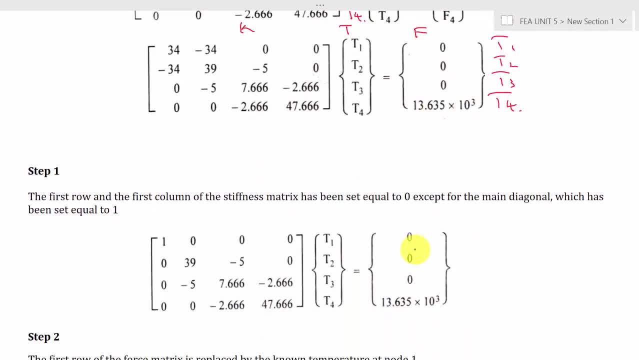 we have to follow four steps. So this is not like the previous case problems, because in the previous problems, that is, in the structural problems, the initial boundary values will not be given, that is, they will not specify any displacement. but here the initial nodal temperature, that is initial boundary condition, is given, so that 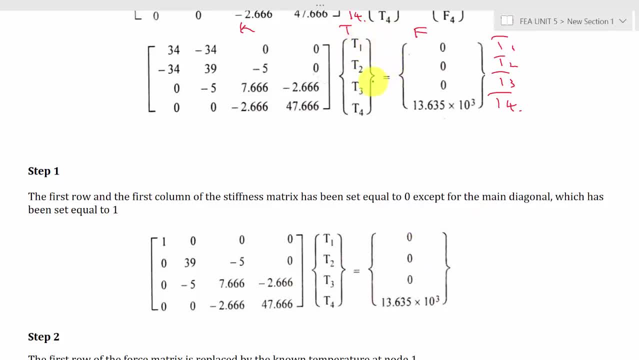 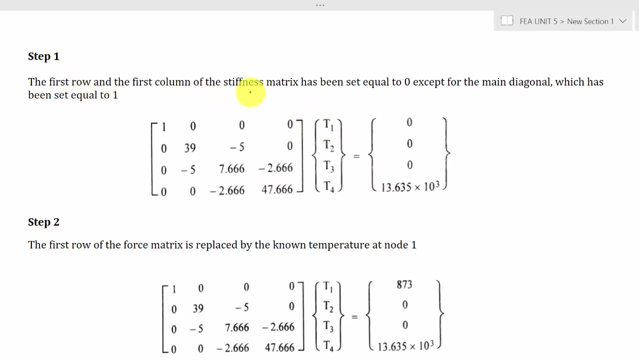 is T1 is given in the problem. so this is called as initial boundary value problems. So for calculating the solution for initial boundary value problems we have to follow some procedures. so now I will tell you the procedure. so first step is the first row and first column of the stiffness matrix has been set equal to 0, except the main diagonal which 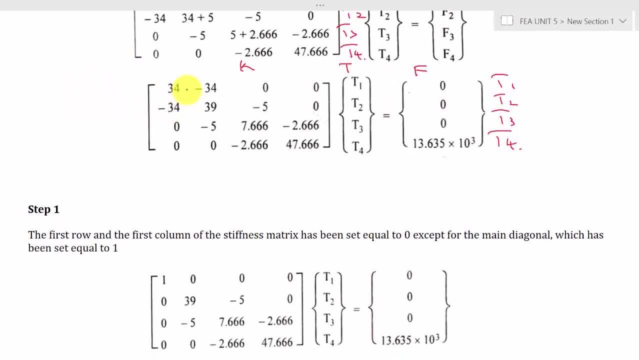 is equal to 1. so here you can see that, except this k of 1,1, the remaining terms are all equal to 0. so here I have replaced this 1,1 by 1 and all the remaining values- that is, first row and first column values- are 0. so this is my step 1 and the step 2 is I am going. 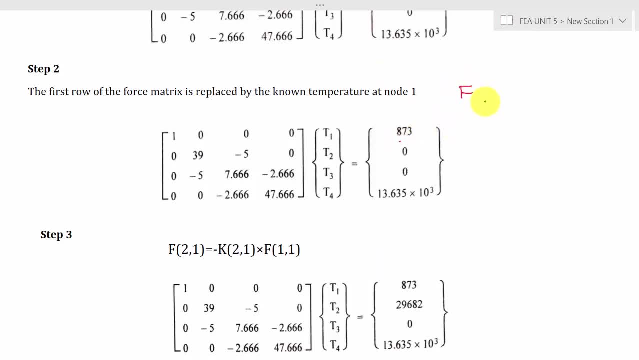 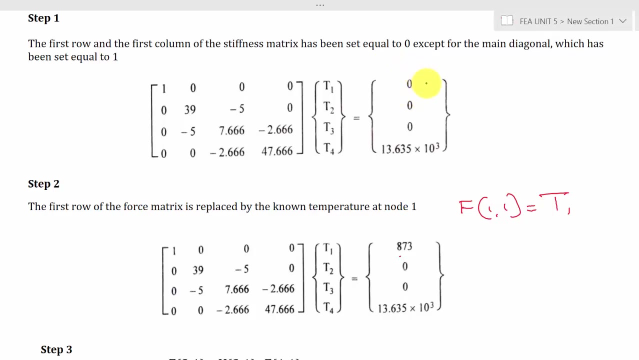 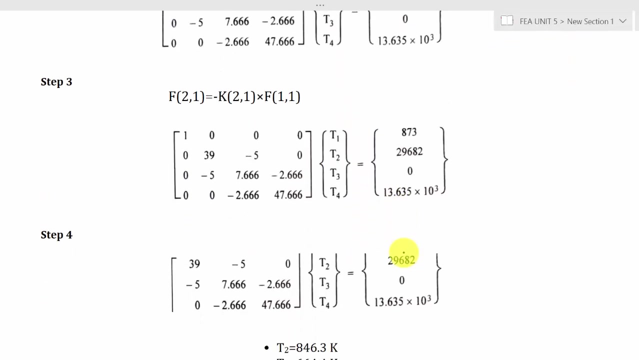 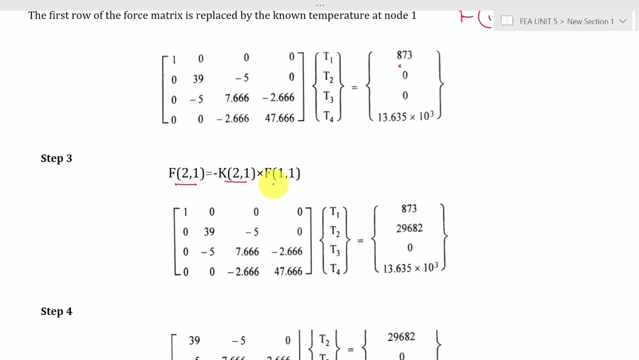 to replace this f of 0.. 1,1 by the known temperature, because I already know the value for T1, that is 873 kelvin. so here I have replaced this first column of first row of force vector by the known temperature. then the third step is: my f of 2,1 is equal to minus of k of 2,1 into f of 1,1. so here: 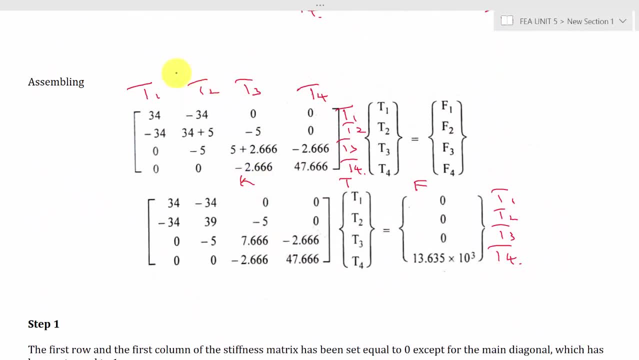 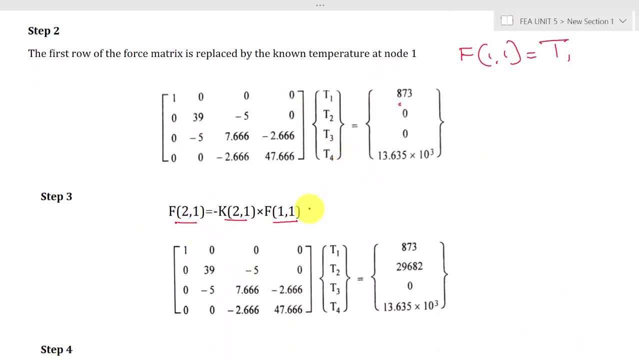 minus of k of 2,1 into f of 1,1 is equal to minus of k of 2,1 into f of 1,1. so here minus k of 2,1 means this is my k 2,1. so that is 34, so here it is equal to. already I have a. 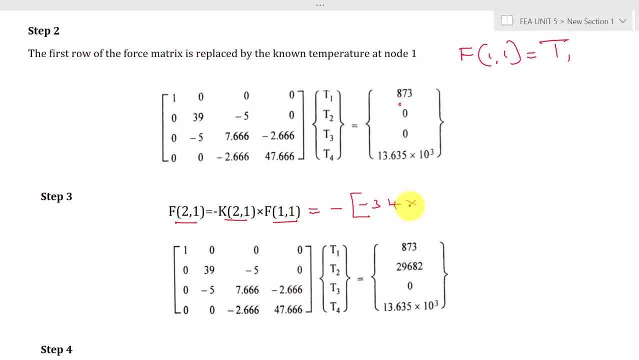 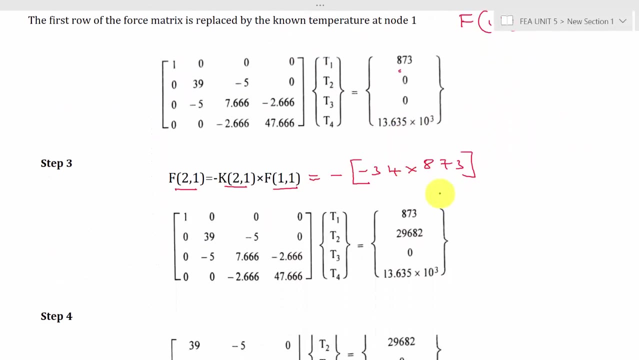 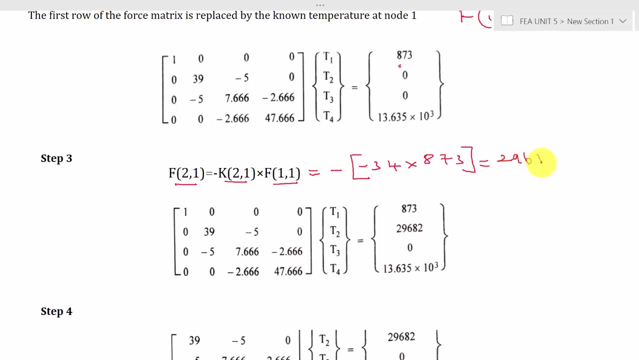 minus. so the value is minus 34 into f of 1,1 is 873. so this step is very, very important. so k of 2,1 is minus 34 into the known temperature 873.. ok, so that is equal to minus and minus will get cancelled. I will get 29682. 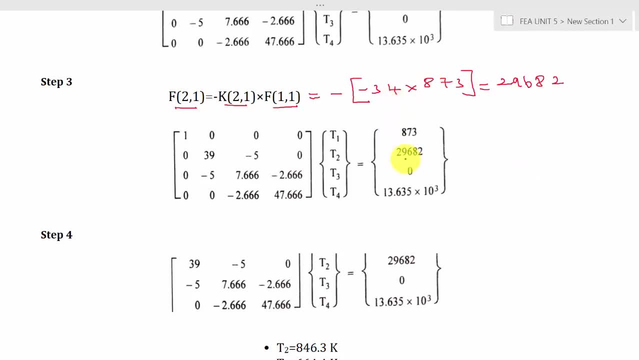 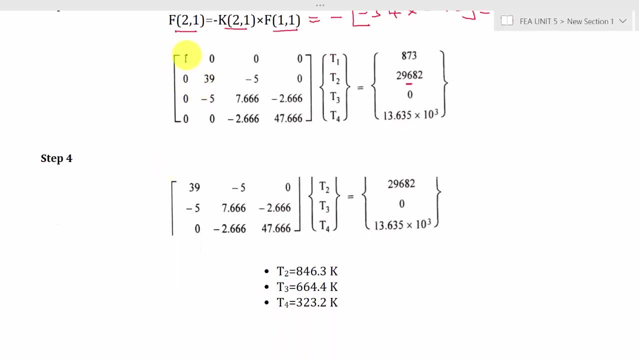 ok, so now I am replacing this f of 2,1 by this calculated value. now I can neglect the first row and the first column of the matrix. so I can neglect this first row and the first column and I can take only the remaining terms. so that is, you will. 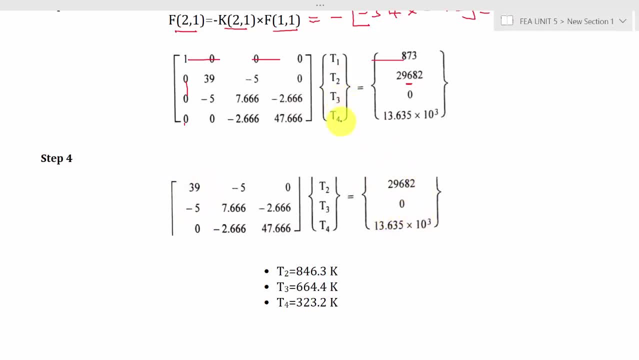 get a 3 cross 3 matrix with t2t3 and t2t3.. ok, so it is equal to minus and minus 1.. Now you can use the calculator to find out the solution. So the final value is: T2 is equal to 846.3 Kelvin, T3 is 664.4 Kelvin and T4 is 323.2 Kelvin. 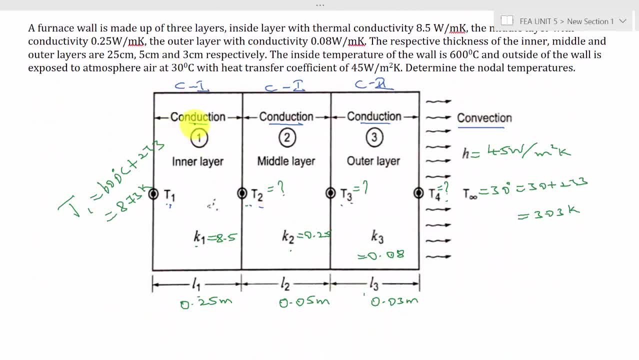 So here we have three elements. First element is subjected to only conduction. that is why it is case 1.. The second element is also subjected to only conduction, so it is case 1.. The third element is subjected to conduction as well as the end convection, so it comes under case 2.. 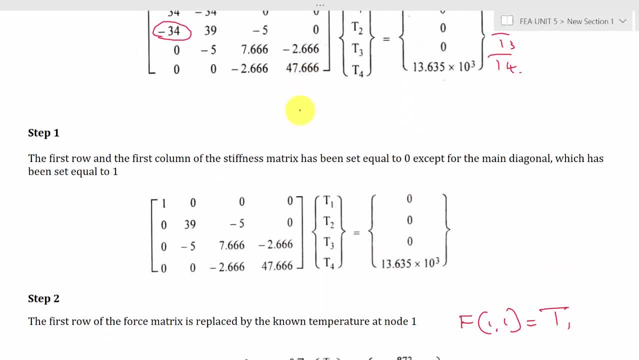 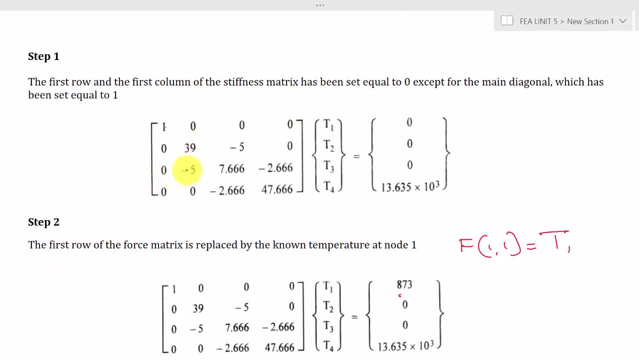 So we can calculate the stiffness matrix individually and we can assemble it After assembling follow the procedure. First step is 1 and the first row and first column values will be 0. Then the second step is: F of 1,1 is equal to the known temperature. 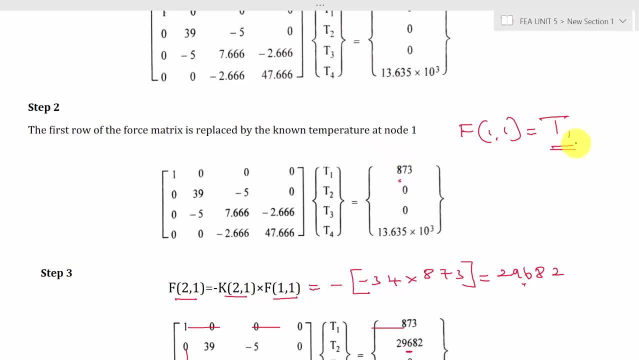 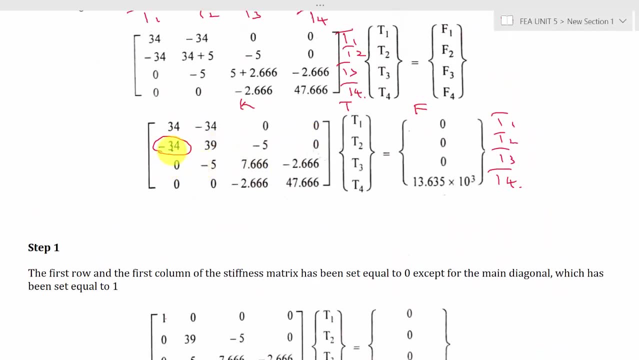 So this T1 value is given in the problem And the third step is: F of 2,1 is equal to minus K of 2,1.. So this is my K matrix: K of 2,1 is minus 34 into the F of 1,1, that is 873.. 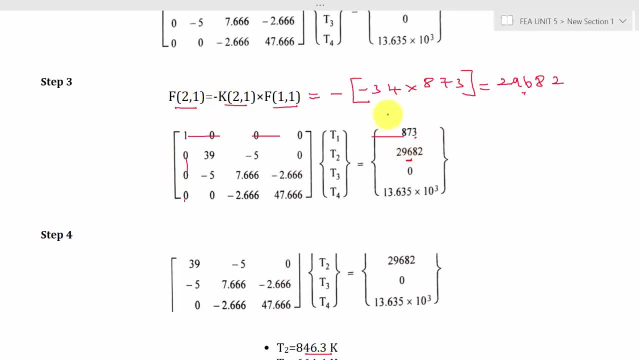 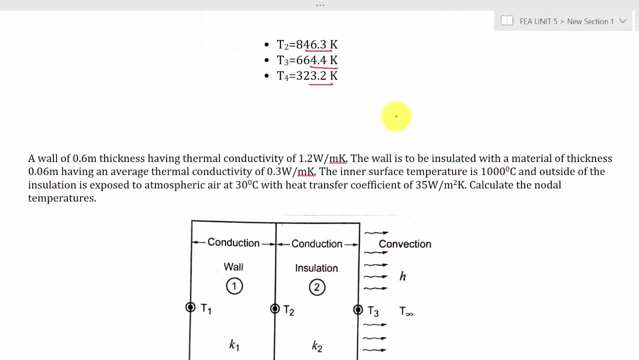 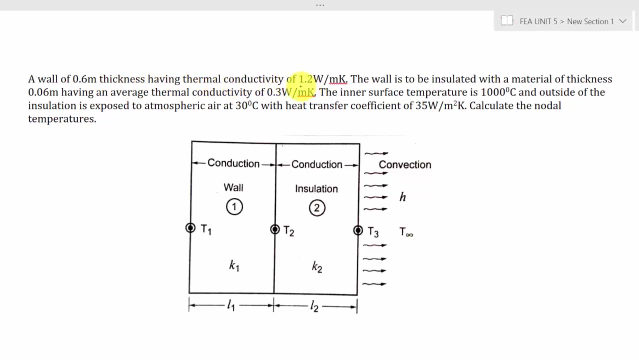 So here I have replaced it. Then you can neglect the first row and first column and you can find out the solution. So this is how we have to approach the one dimensional heat transfer problems. So this is the tutorial problem: A wall of 0.6 meter thickness having thermal conductivity of 1.2 watt per meter Kelvin.